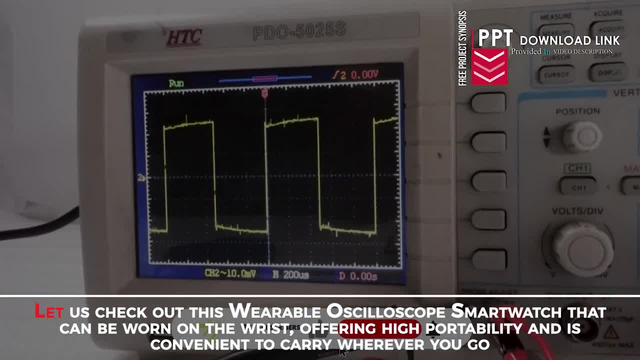 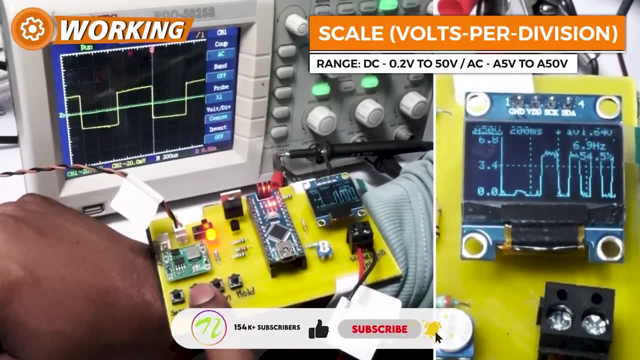 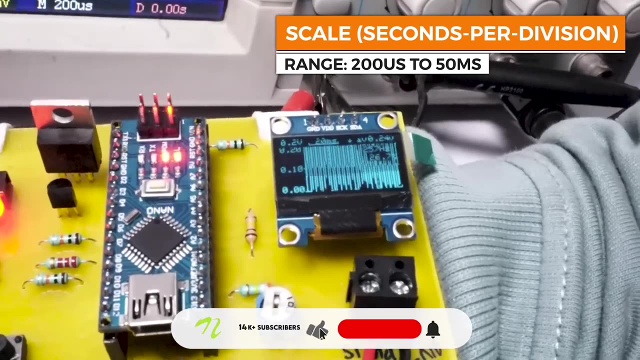 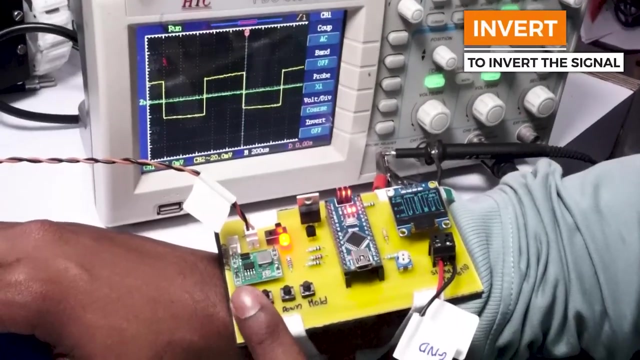 oscilloscope smartwatch that can be worn on the wrist, offering high portability, and is convenient to carry wherever you go. A very capacious size can be worn for long periods and is likely to carry long periods of time when worn. This is a smartwatch that is fit for a large 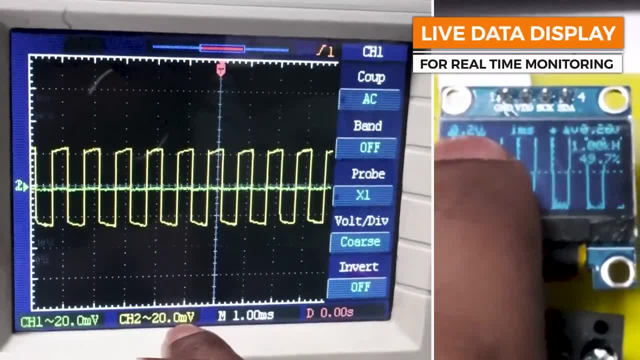 home and will provide a good grip. 12. Smartwatch: Smartwatches are not only for a short time. the smart watch can even be held in the hands of your family. They can also be used for a period of time and while not only at start and end of the day. but at the end of the day, they can also be used as part of daily trips, such as when you are on the road or at a bike race. Smartwatches are a mere piece of hardware and are often prepared to be equipped with the necessary 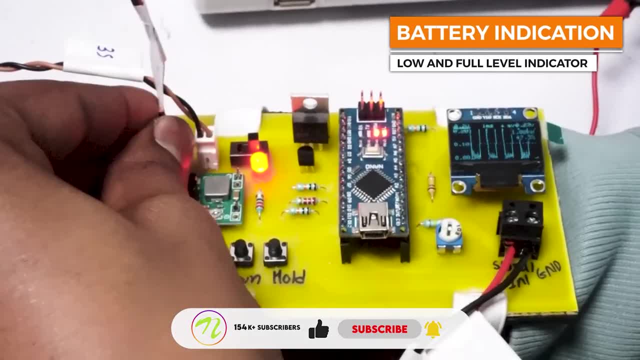 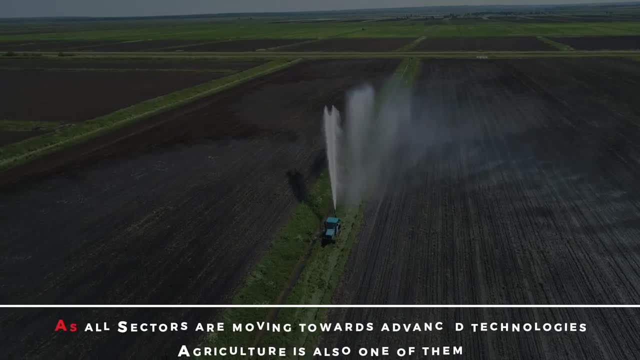 equipment for greater reliability and security. The smartwatch is an extremely portable smartwatch with a great handle. The smartwatch battery is available in $50,000, and is available at a price of $100,000, including Solar Seed Sprayer Robot. 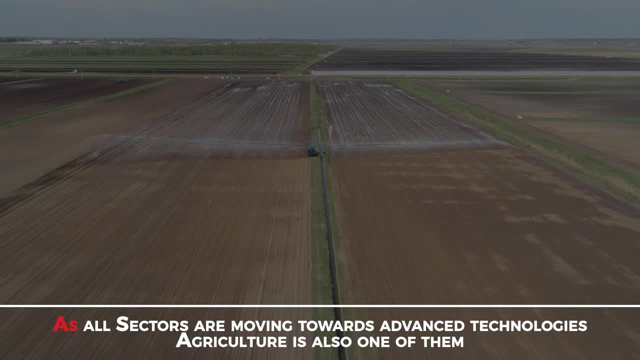 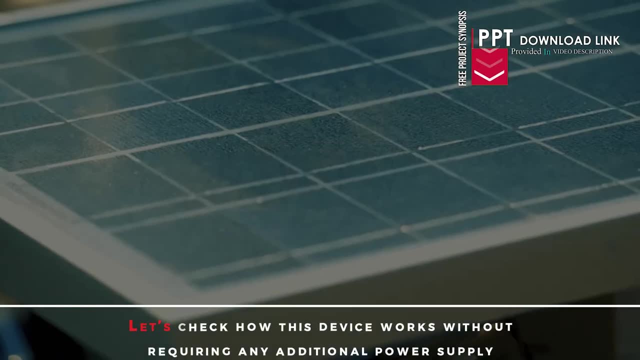 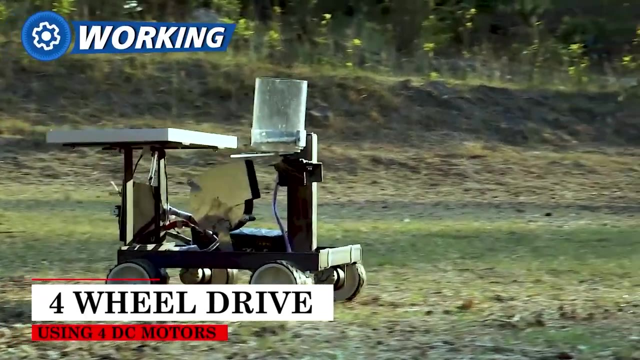 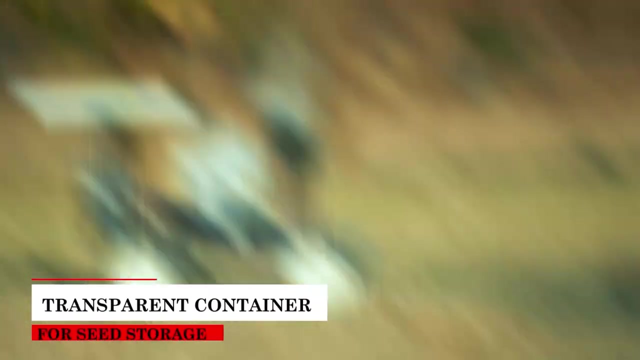 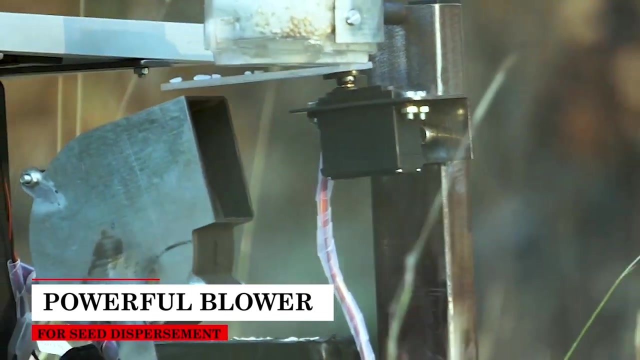 As all sectors are moving towards advanced technologies, agriculture is also one of them. Using a solar-powered seed sprayer robot, the process of seed sowing becomes easier and more convenient. Let's check how this device works without requiring any additional power supply. 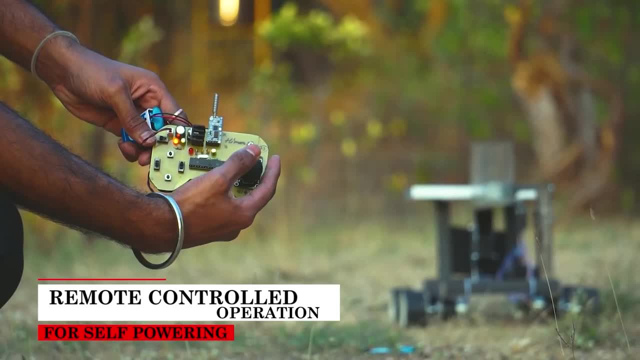 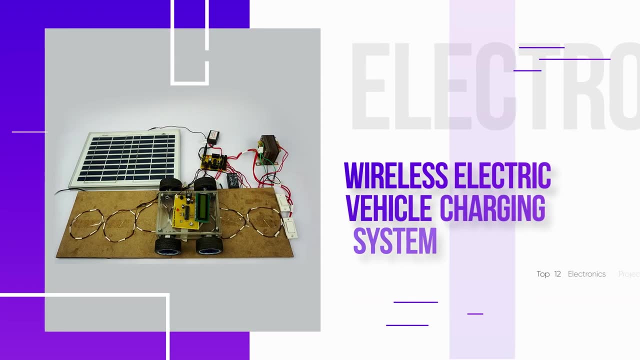 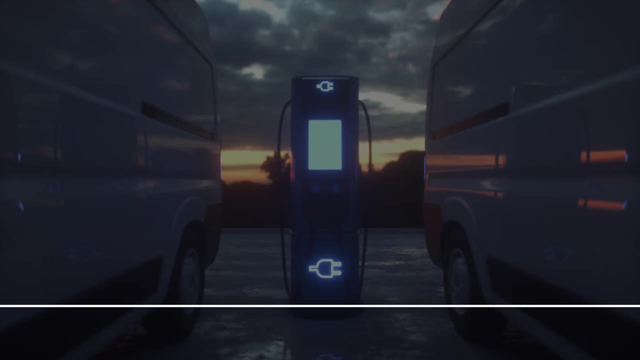 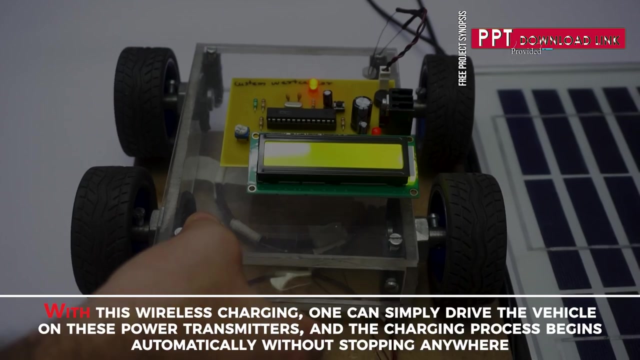 Let's go. Wireless Electric Vehicle Charging System Using charging cables and plugs require manual connection and disconnection of a vehicle from the charging station. This process can be less convenient, especially in bad weather conditions or if the charging station is fully occupied. With this wireless charging, one can simply drive the vehicle on these power transmitters. 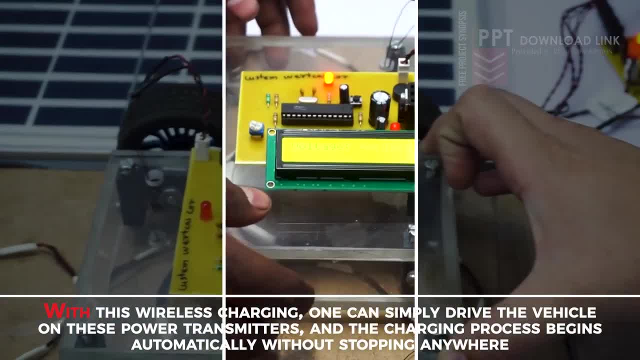 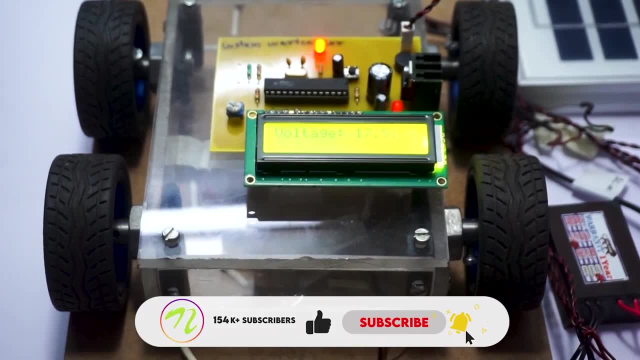 and the charging process begins automatically without stopping anywhere. So, using this mechanism, the vehicle, when it moves over the road, it does not need to stop for charging and it is charged continuously as it goes over the road. So these coils are connected to a transformer, which is used to power them. 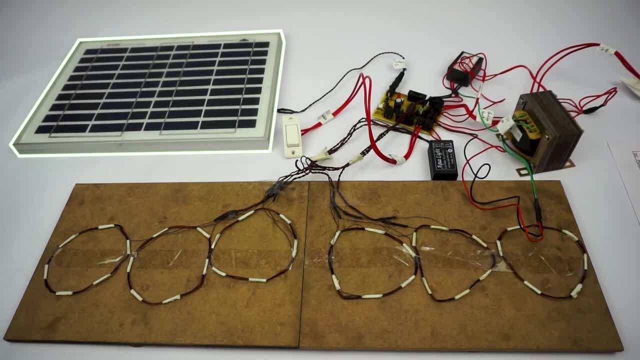 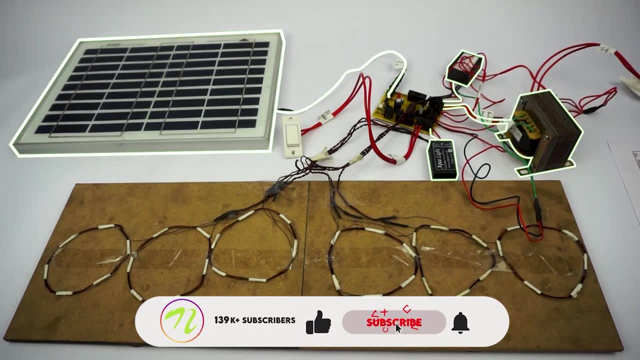 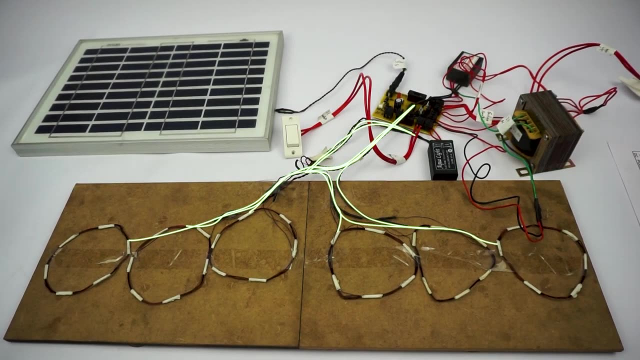 How basically the system works is the solar panel you can, as you can see here, is used to charge the battery using charge controllers. So the charge from the battery is converted to AC power using the transformer, because for wireless transmission we need the power to be AC power. and after the power is transmitted, 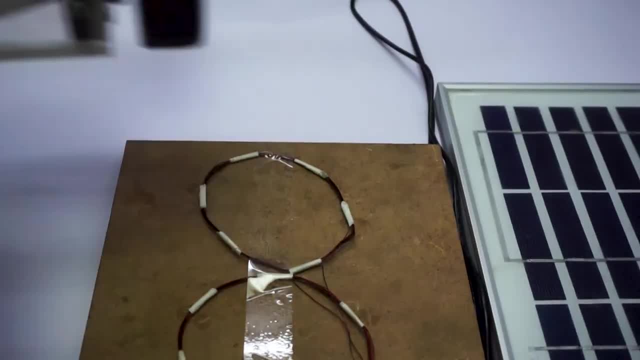 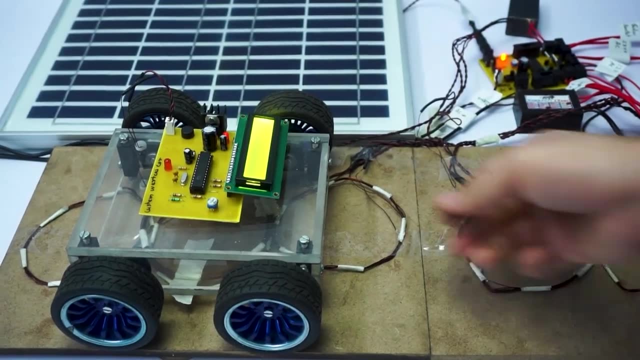 from the coils on the road, It is received by the coil underneath the vehicle and this perceived power is again converted into DC so that it can be used to charge the vehicle battery. So now let's move the vehicle over the track and, as you can see, as it moves over the road, 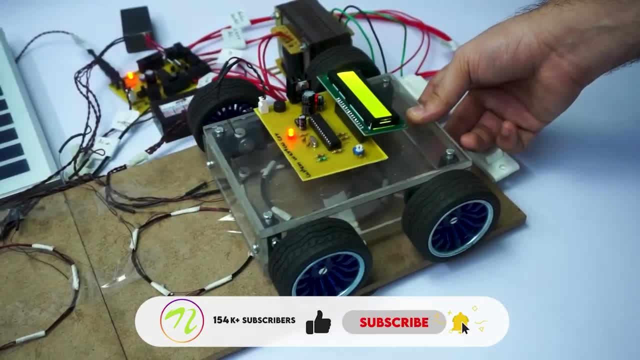 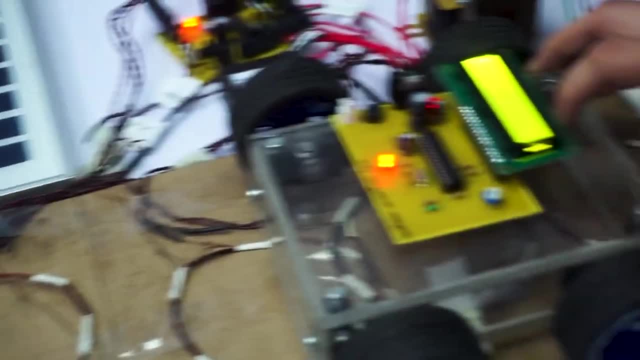 the power is transferred wirelessly to the circuit and, as you can see, the box of the vehicle is made to be transparent and the coil that is mounted inside the vehicle is used to power the vehicle circuit and also show the voltage generated. So here we can see the voltage. 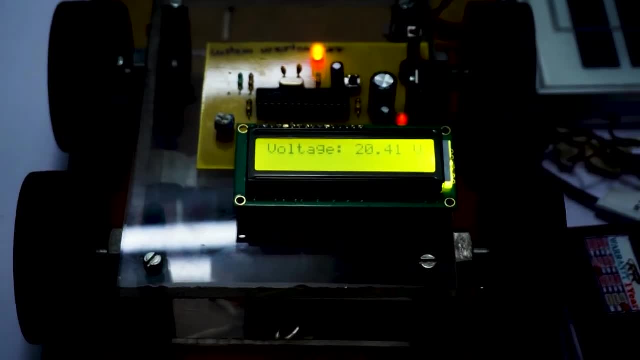 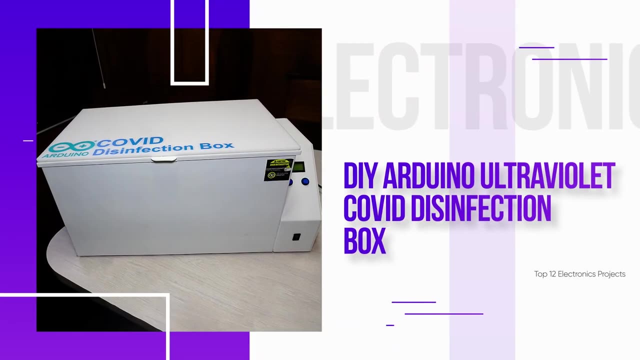 The voltage that is generated received at the vehicle and as it moves over the road. So this is how the system works: DIY Arduino Ultraviolet COVID Disinfection Box. Due to the fast and efficient spread of COVID, we could wear face masks and gloves to protect. 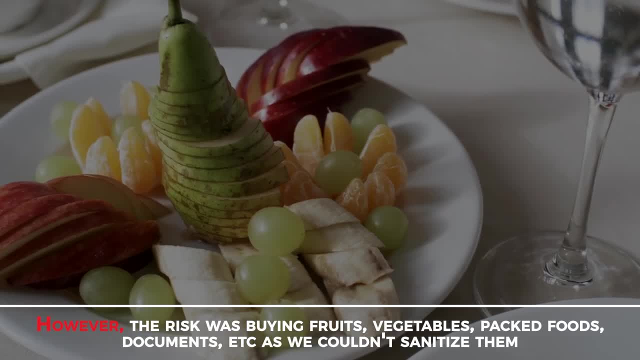 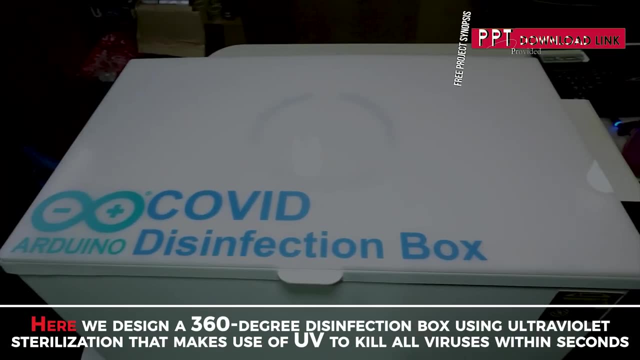 ourselves from everything we touched. However, the risk was buying fruits, vegetables, packed foods, documents, etc. as we couldn't sanitize them Here, we designed a 360-degree disinfection box using ultraviolet sterilizers. We were initially interested in the appearance of the dongle box. 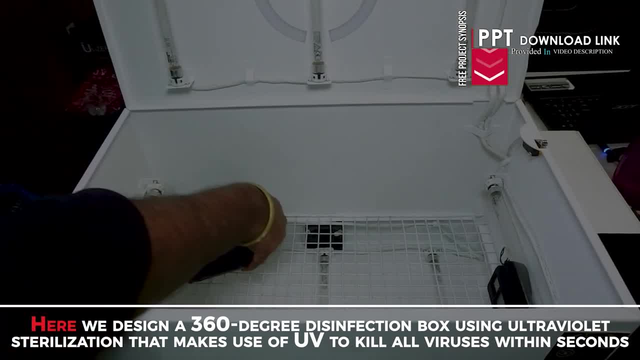 We decided to use this for a special purpose that was used for disinfection purposes. We were also interested in the possibility of putting a dongle box on the front seat of our car. That was our first purchase, But even after the dongle box was made, we were also interested in the function of the 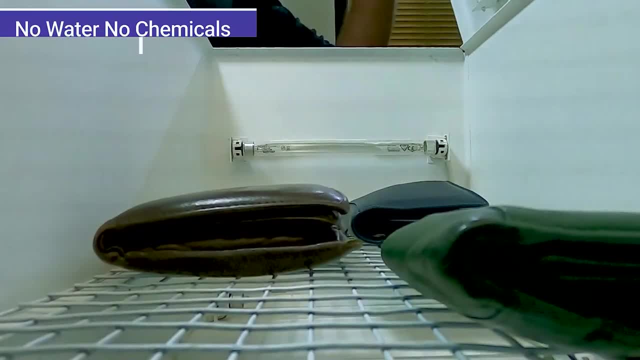 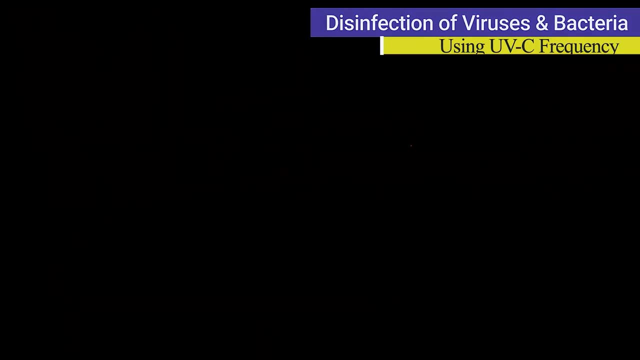 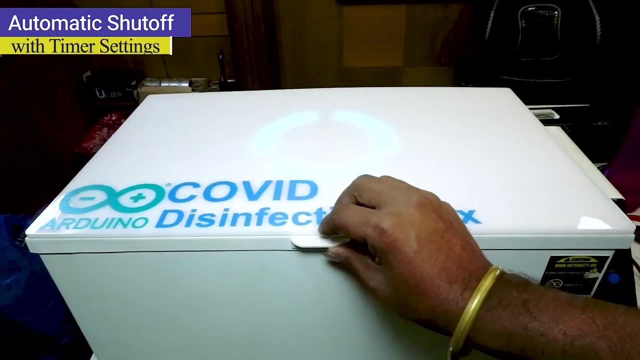 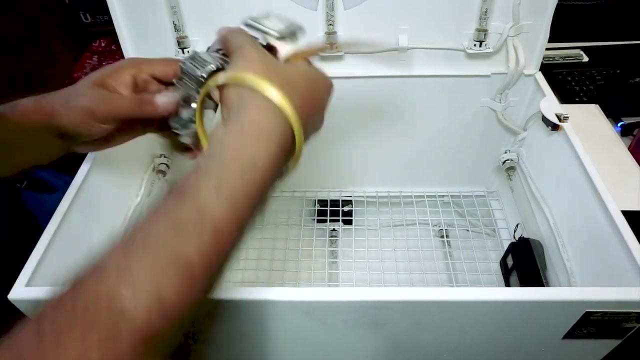 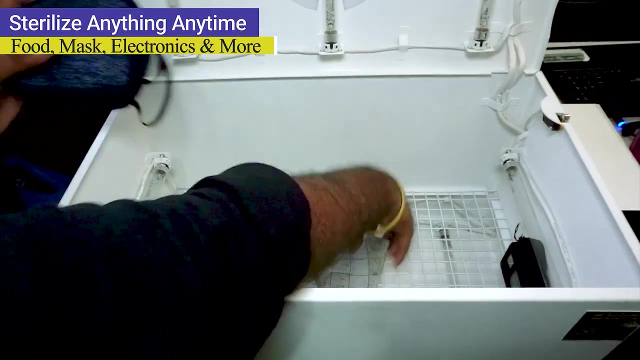 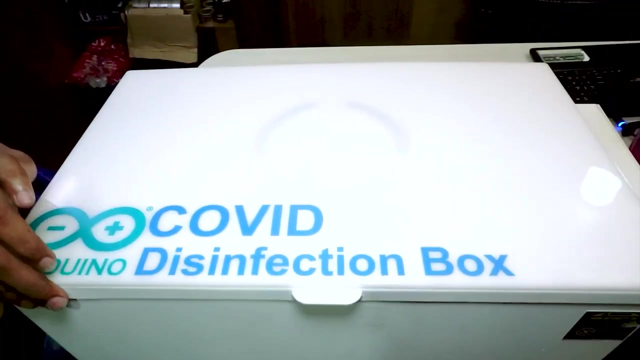 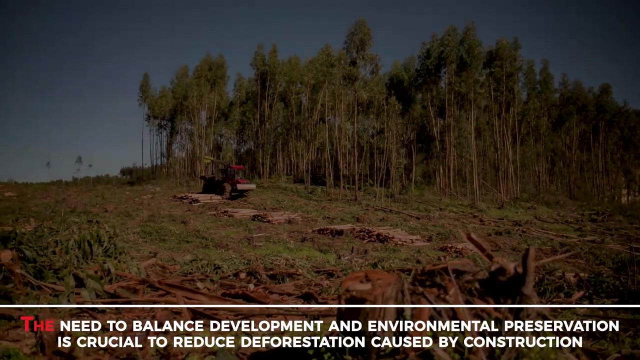 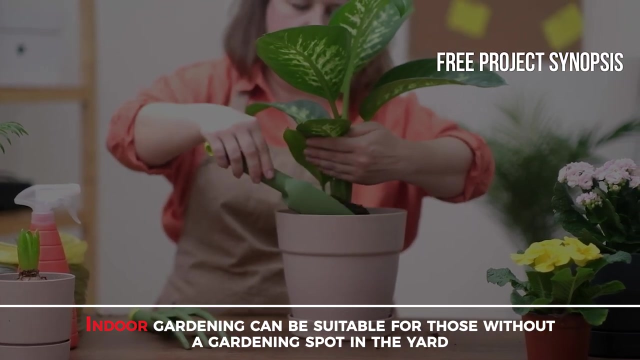 dongle box and how it could be processed, So we decided to use a device to get our Antiochian Indoor Hydroponic Plant Grow Pot. The need to balance development and environmental preservation is crucial to reduce deforestation caused by construction. Indoor gardening can be suitable for those without a gardening spot in the yard. 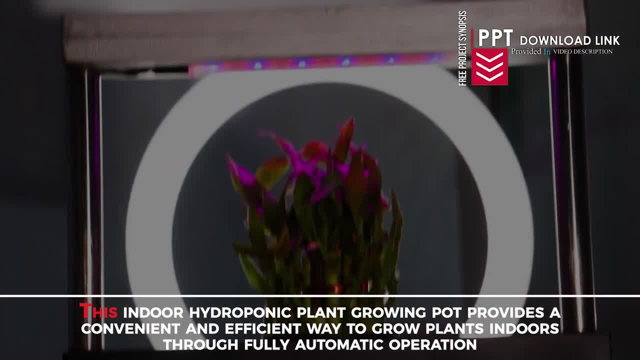 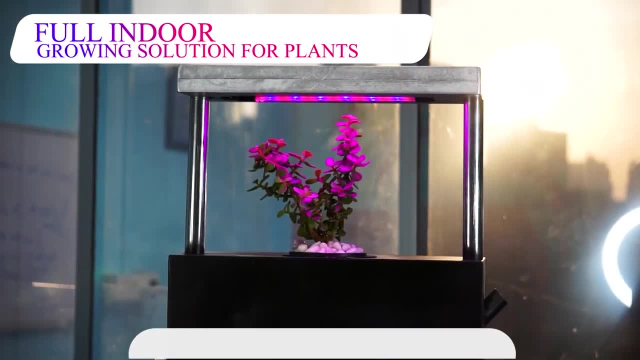 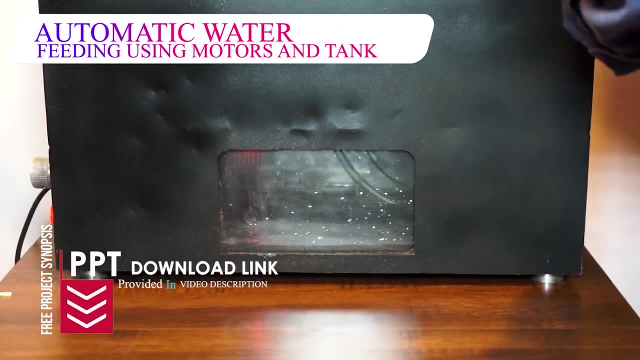 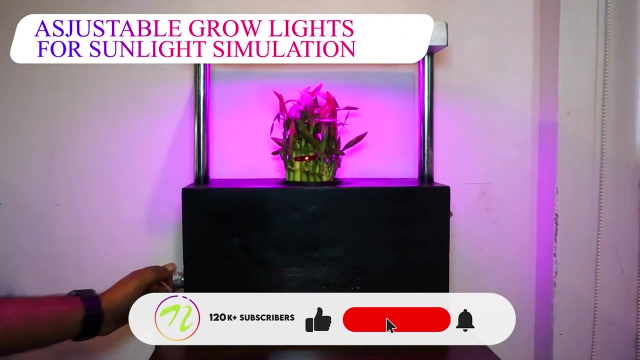 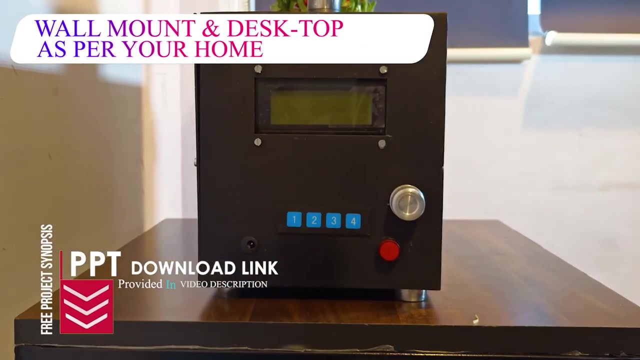 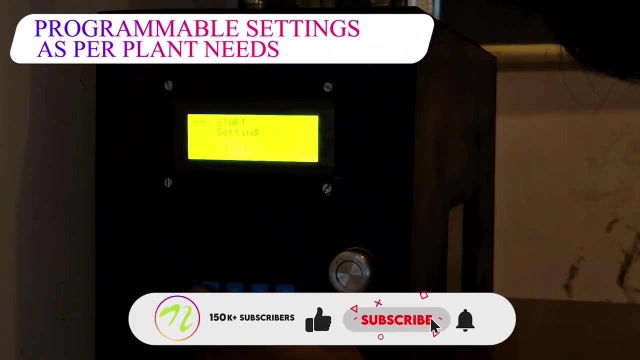 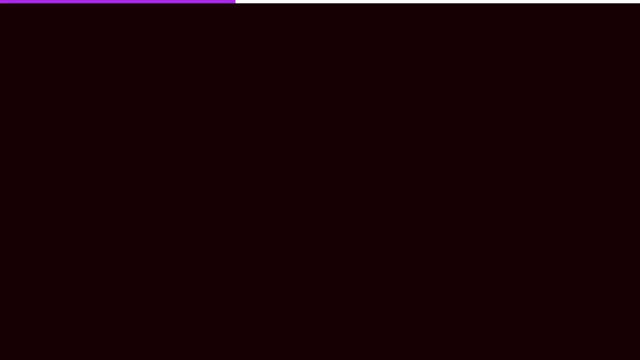 This Indoor Hydroponic Plant Grow Pot provides a convenient and efficient way to grow plant indoors. through fully automatic operation, Ongoing positive effects of Indoor Hydroponic Plant Grow Pot can be reduced to take out all dust and debris from plants, causing good soil moisture. 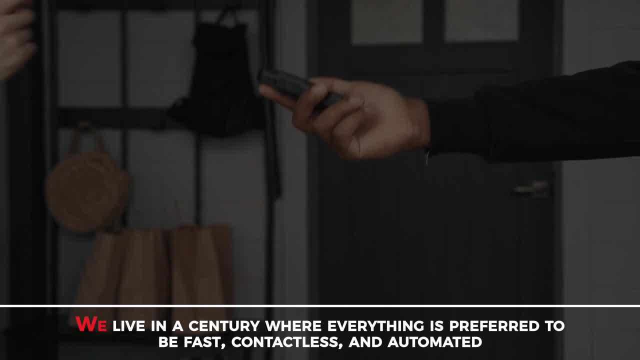 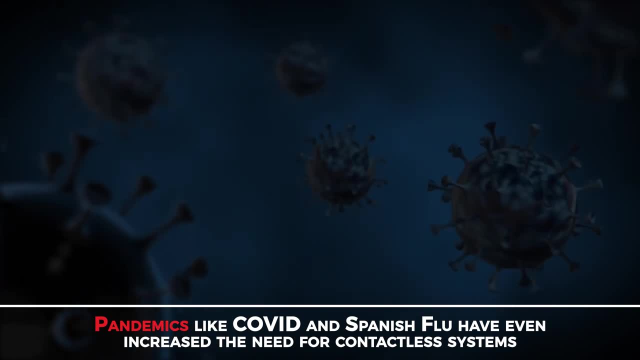 Contactless IoT Doorbell. We live in a century where everything is preferred to be fast, contactless and automated. Pandemics like COVID and Spanish flu have become so common for all of us that now we and the Spanish Flu have even increased the need for contactless systems. 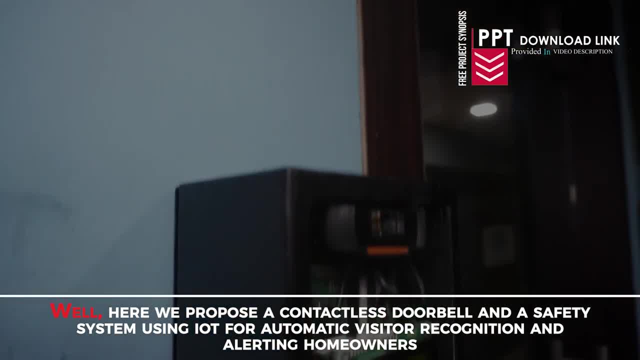 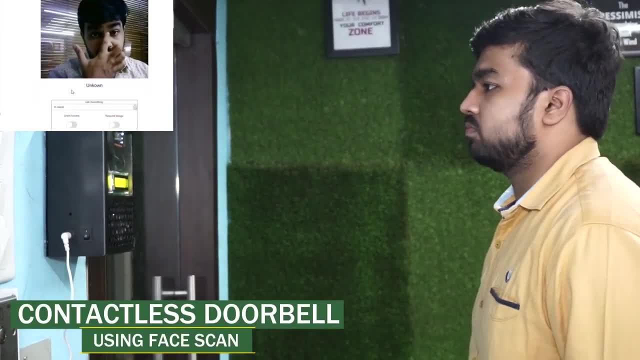 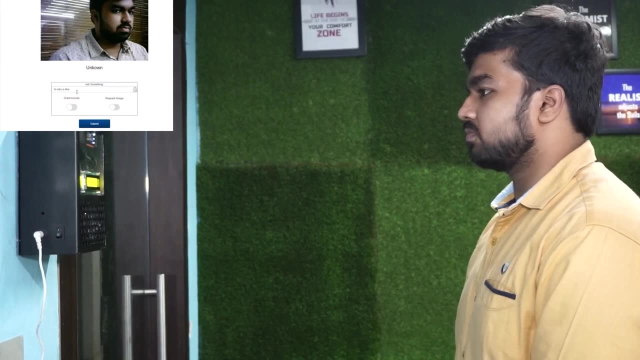 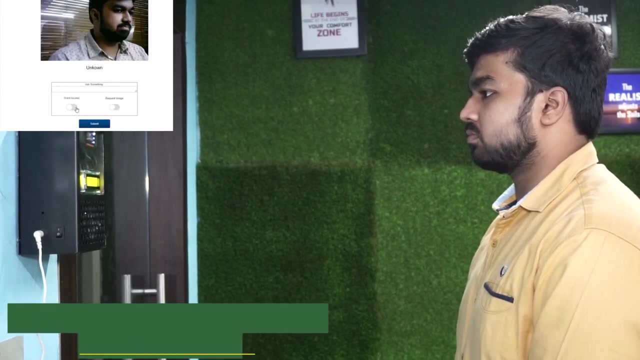 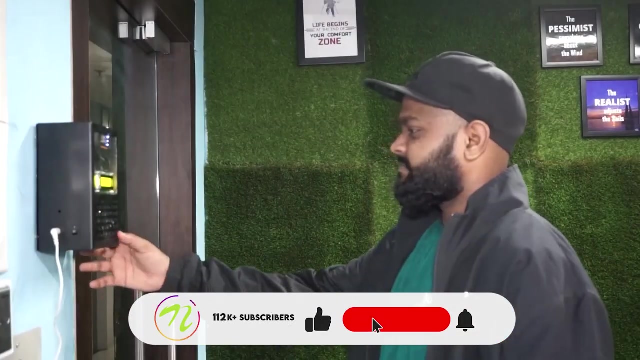 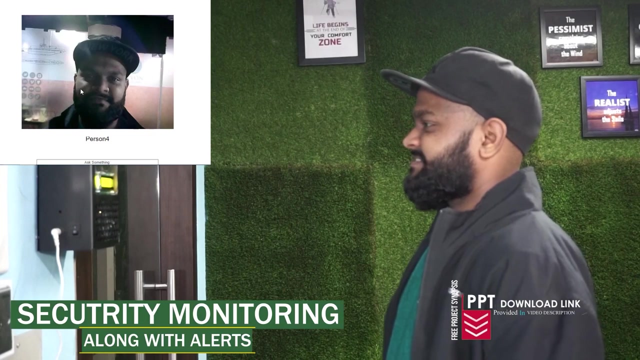 Well, here we propose a contactless doorbell and a safety system using IoT for automatic visitor recognition and alerting homeowners For需要. to invest ourselves and in our customers, we unite in the Not- навarigo向 el tibio COVID-19 Chips. 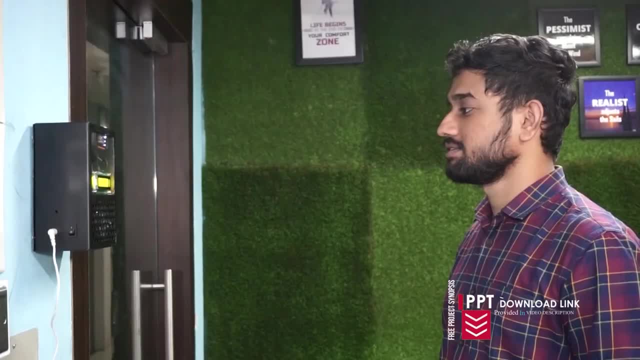 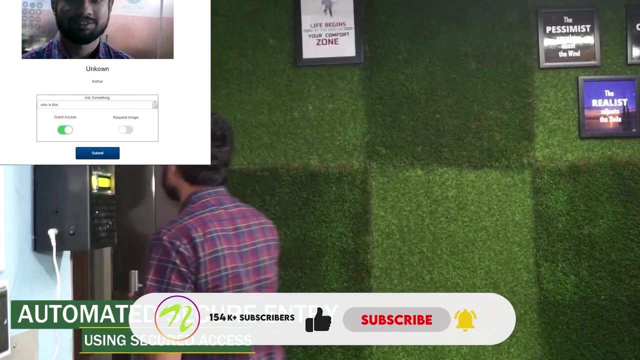 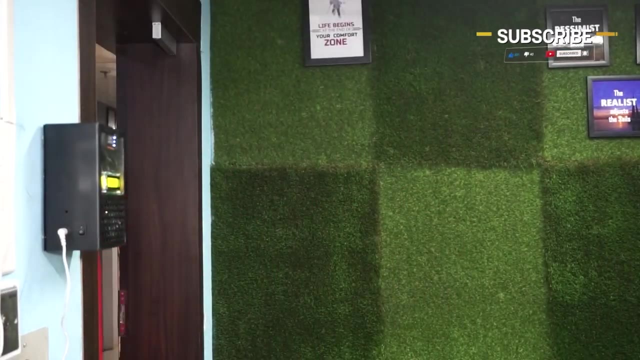 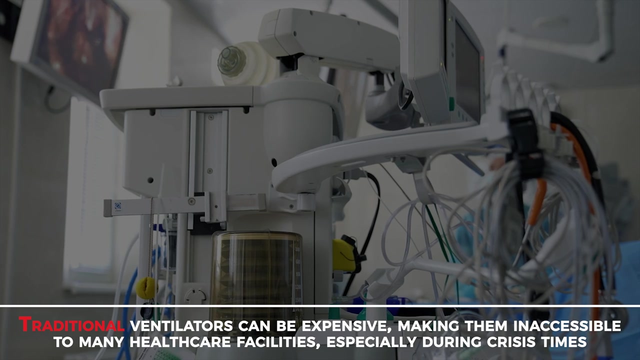 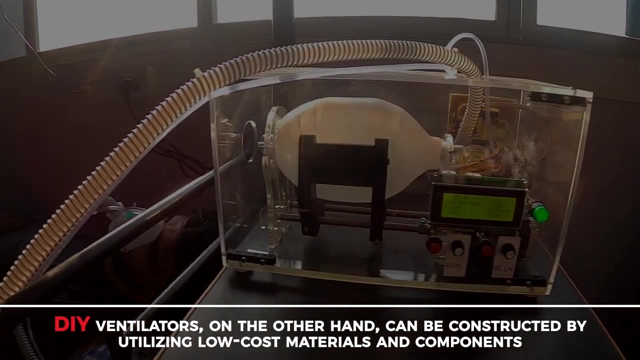 Our FMN American Department of 노동 nada me, I me. DIY, low cost ventilator. Traditional ventilators can be expensive, making them inaccessible to many healthcare facilities, especially during crisis time. DIY ventilators, on the other hand, can be constructed by utilizing low cost materials. 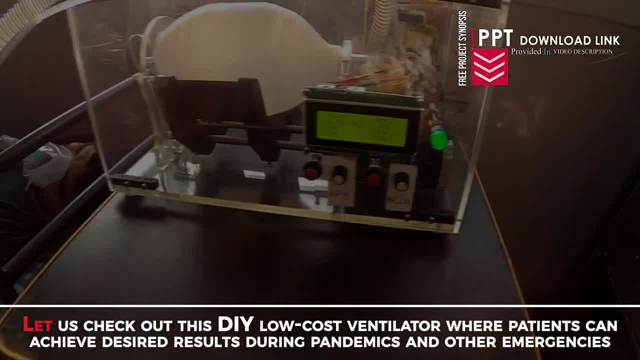 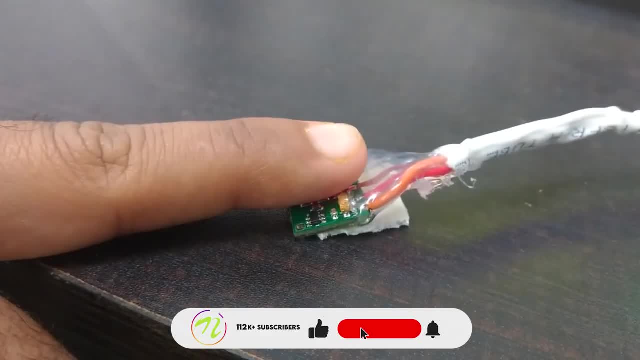 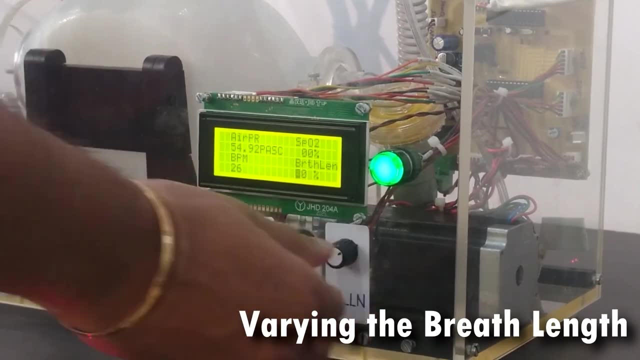 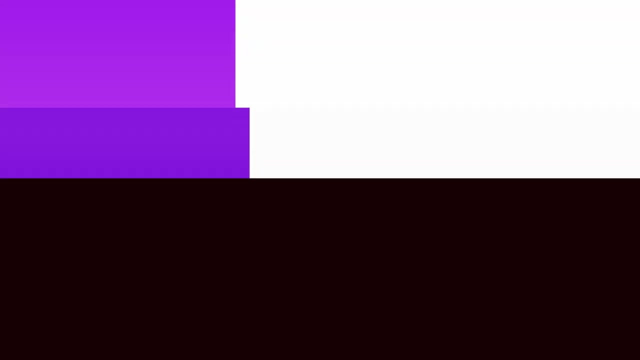 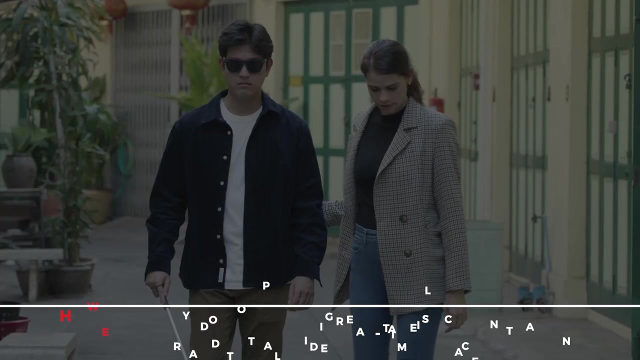 and components. Let us check out this DIY, low cost ventilator where patients can achieve desired results during pandemics and other emergencies. GPS Tracking- Blind Stick. Blind walking sticks can only detect obstacles that physically touch them. However, they do not provide real-time location tracking or additional navigation. 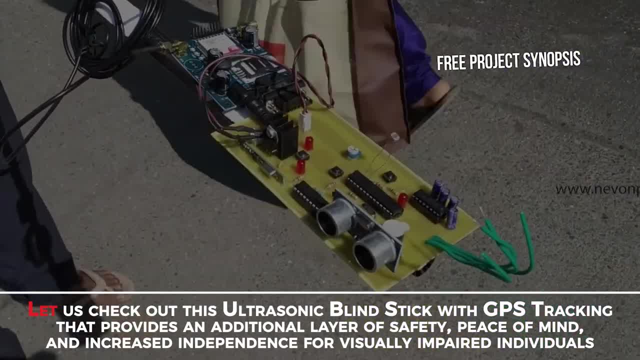 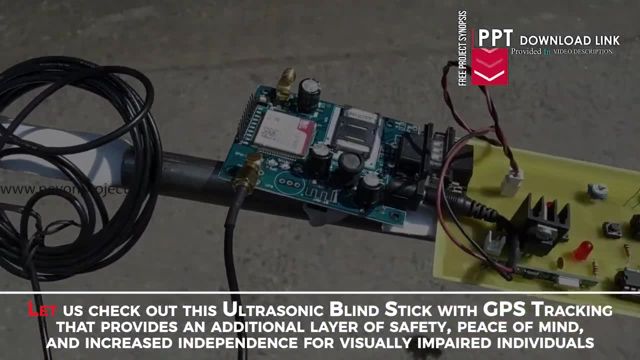 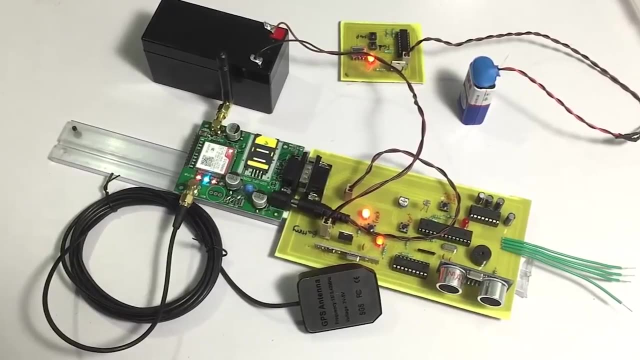 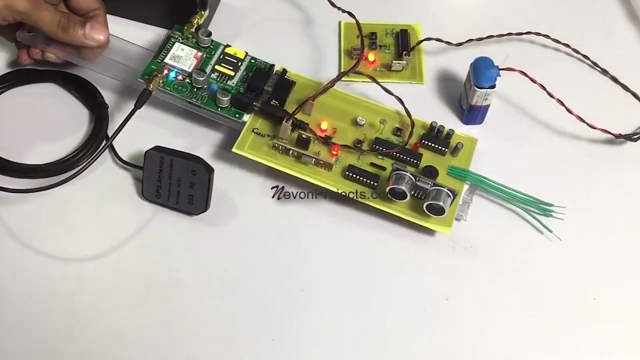 assistance. Let us check out this ultrasonic blind stick with GPS tracking that provides an additional layer of safety, peace of mind and increased independence for visually impaired individuals. First, we will see how it avoids the obstacles in front of the blind. Suppose we have the blind stick in here and there is an obstacle in front of it. 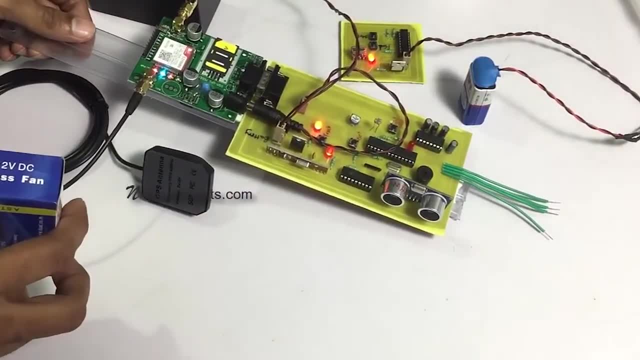 Then it gives this beeping sequence that gives the signal that the blind stick is in front of it. This means that the blind person is in front of it. There is an obstacle in front of the stick, So by hearing this, the blind person can avoid that track. 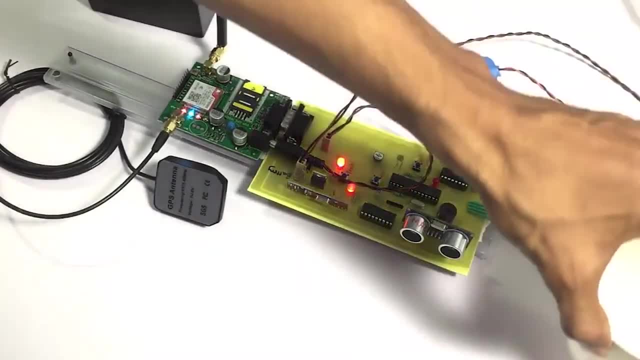 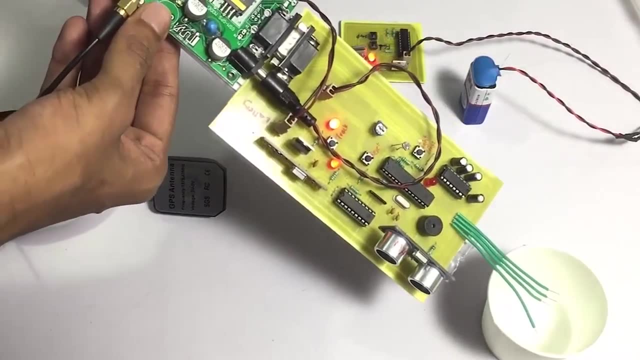 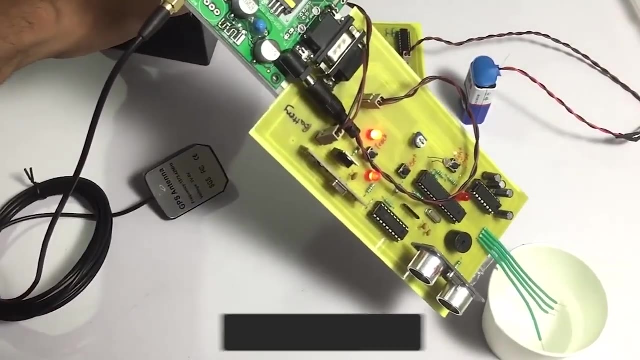 Now let us see places with water. Suppose this is a place where there is water in this glass and the blind person enters that area. So when the stick goes at that point you can see that this beeping sequence tells the blind person that there is a water on in front of him and he should avoid going there. 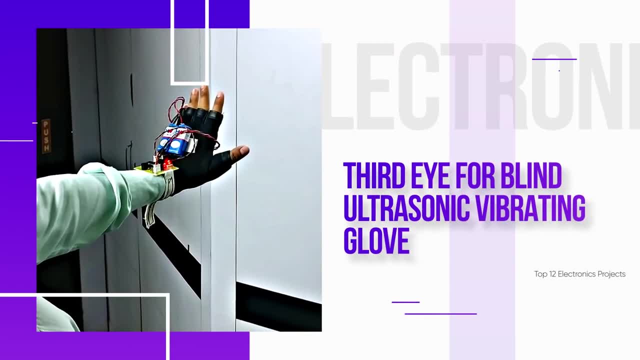 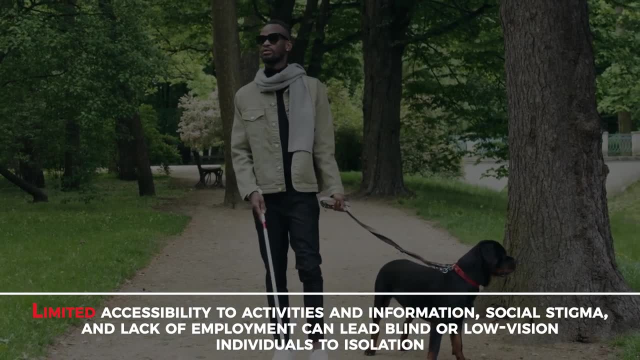 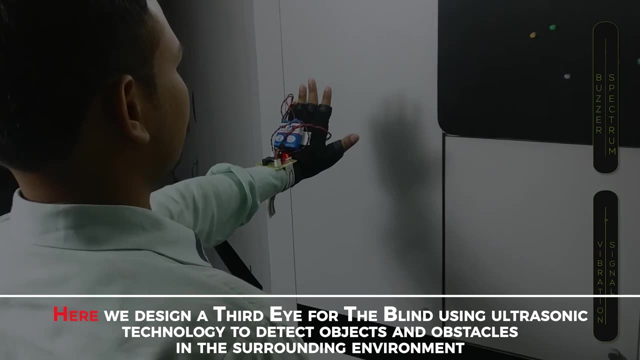 3rd Eye for Blind- Ultrasonic Vibrating Glove. Limited accessibility to activities and information, social stigma and lack of employment can lead blind or low vision individuals to isolation. Here we design a 3rd eye for the blind, using ultrasonic technology to detect objects and obstacles in the surrounding environment. 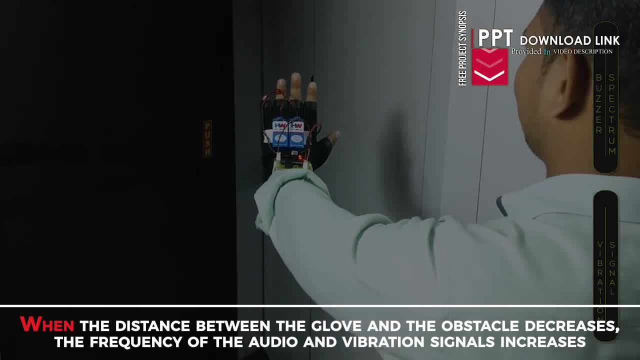 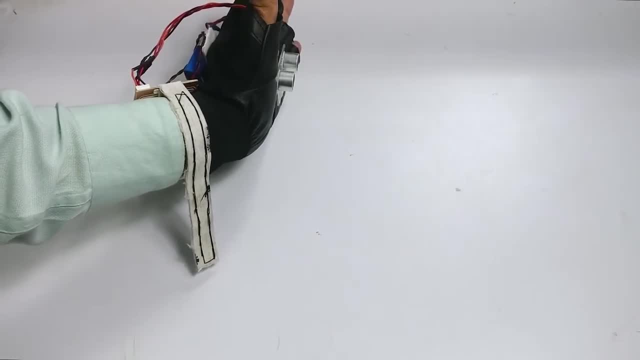 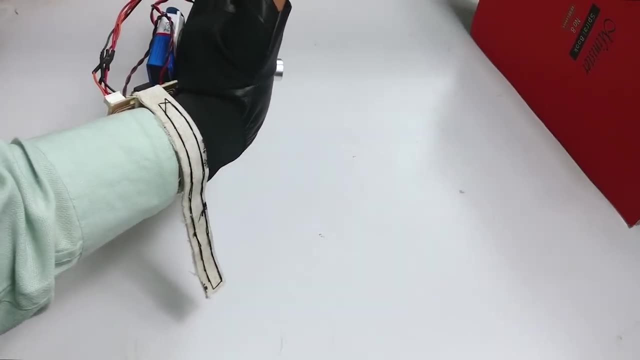 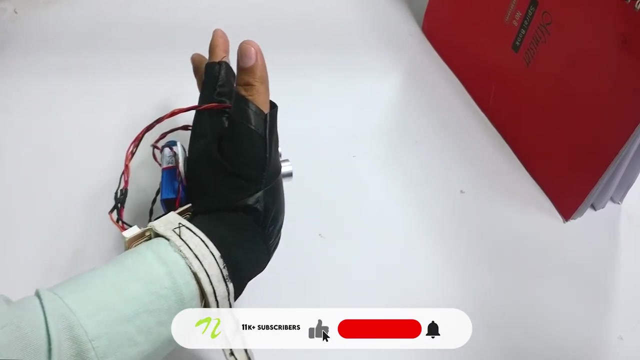 When the distance between the glove and the obstacle decreases, the frequency of the audio and vibration signal increases. Assistive, additional and Readiness Content. Digital schoolbell. With a digital schoolbell, the entire school will be able to perform its non-standard tasks without any inconvenience. 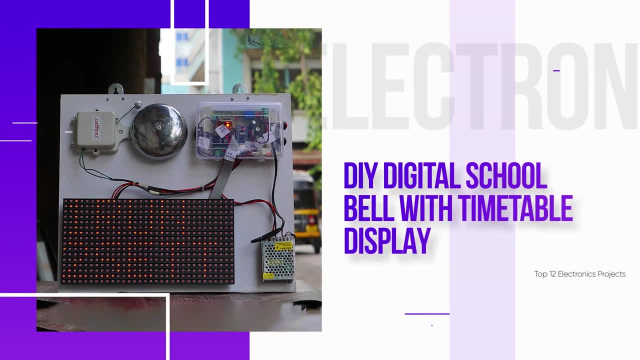 • DIY Digital School Bell with Time Table Display. With the advent of technology, many things have been digitalized, but the school bell remains manual. • DIY Digital School Bell with Time Table Display. With the advent of technology, many things have been digitalized, but the schoolbell remains manual.